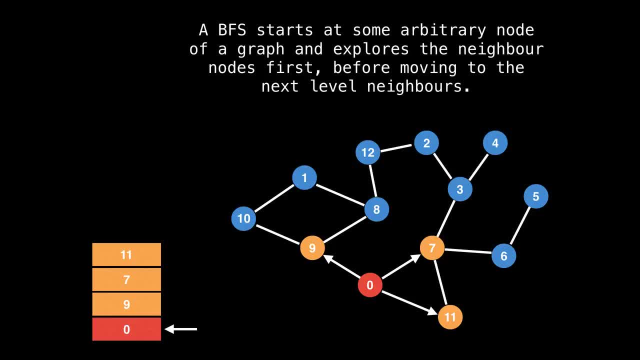 zero has no more unvisited neighbors. So we move on. So nine is next up in the queue. So we add all of nines unvisited neighbors to the queue. So that is 10 and eight. Then there are no more neighbors of nine to visit. So we move on to the next node in our queue. 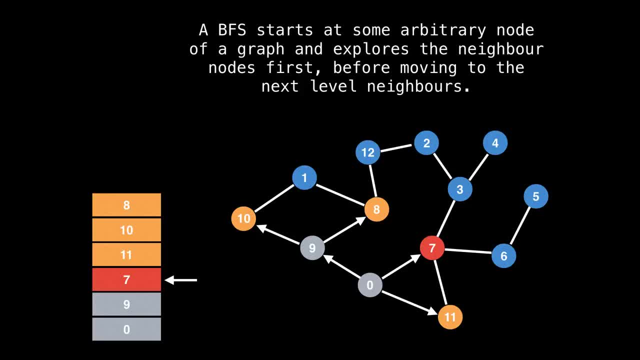 which is seven. then we add all of sevens unvisited neighbors to the queue, So we try and visit node 11.. But node 11 is already in the queue So we don't want to add it again, So we skip it. then we would add six to the queue and three. 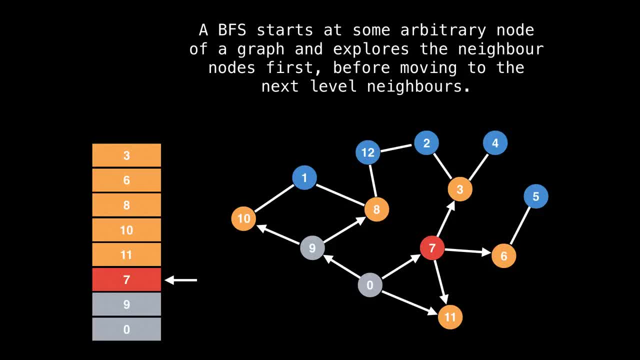 to the queue, And then this process goes on and on until we run out of nodes in the queue. So I will let the animation play. Okay, so, and that's how you do a breadth: first search in a nutshell In the previous animation. 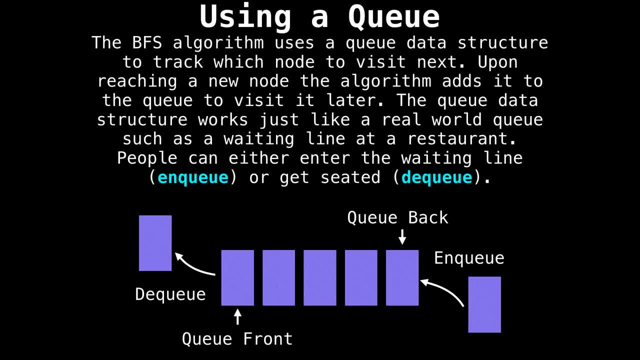 we relied on a queue to help us track which node we should visit next. Upon reaching a new node, the algorithm adds it to the queue to visit it later. The queue data structure works like a real world queue, such as a waiting line in a restaurant. 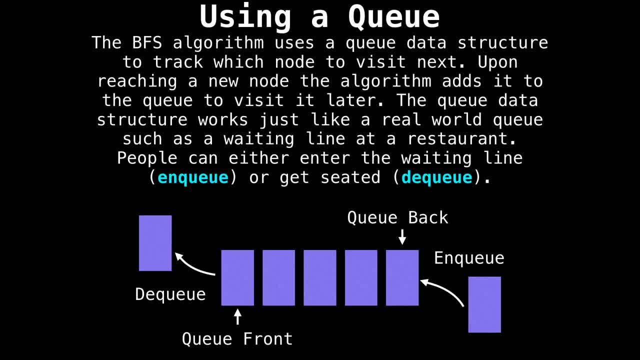 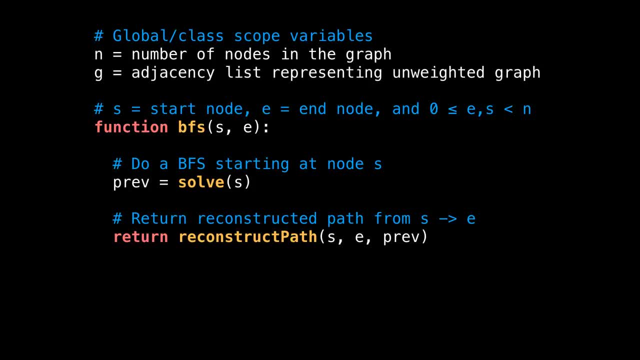 People can either enter the waiting line, that is, get an queued, or get seated de queued. Let's look at some pseudocode for the breadth first, search First things first. we'll need two variables: and the number of nodes in our graph, And G, the adjacency list representing 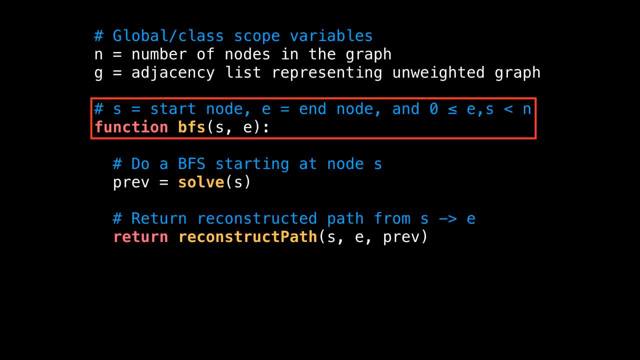 our unweighted graph. This breadth first search function takes two arguments: s and E, the start and end node indices of the search. The return value for this function is the shortest path of nodes from s to E. I've divided the function into two methods for simplicity. 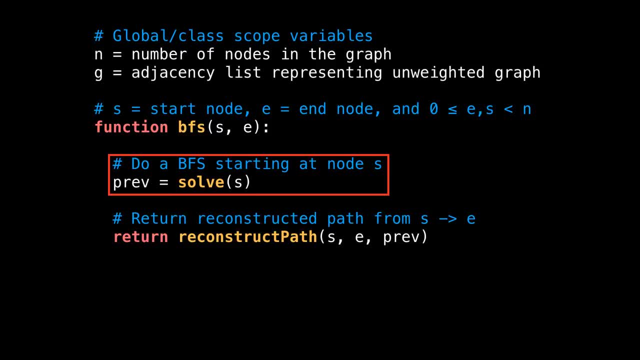 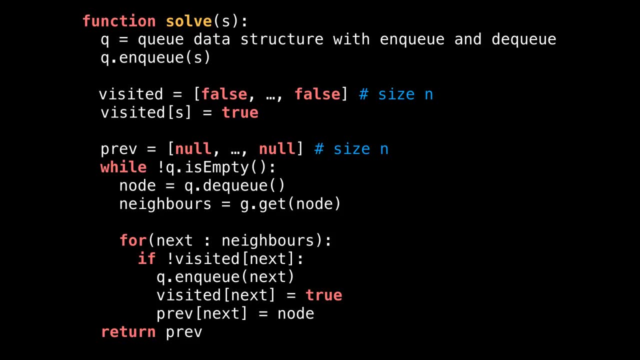 First we solve the problem by executing the breadth: first search and then we reconstruct the path from s to E. So let's take a look at the solve method. So here we are. inside the solve method, The first thing I do is initialize the queue data structure that we'll need and add the starting node. 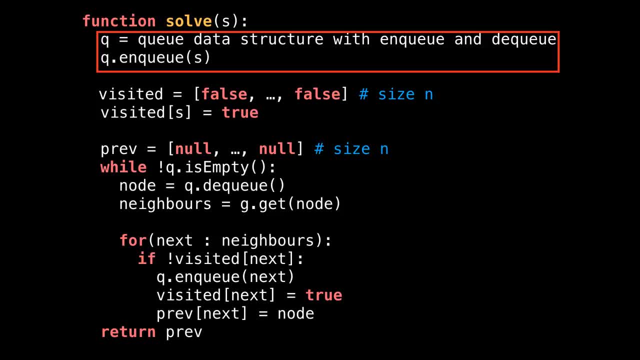 to it. This queue should support at minimum the end queue and dequeue operations I just talked about. then initialize a Boolean array with all false values and mark the starting node as visited. This array tracks whether or not node I has been visited If the value 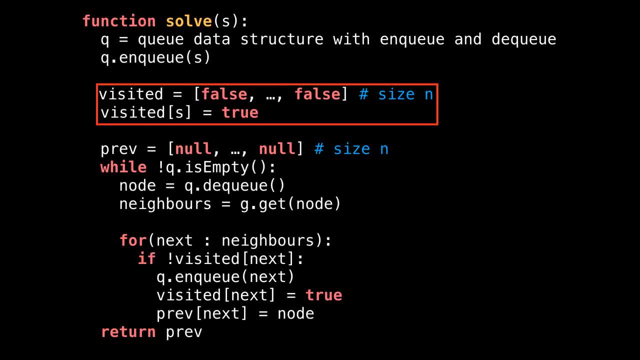 at index i is true, then the node has either been visited or is being visited and is on the queue And the animation. this corresponds to the gray and yellow nodes. The last thing we'll need is an array called Prev, which will help us reconstruct the shortest path. 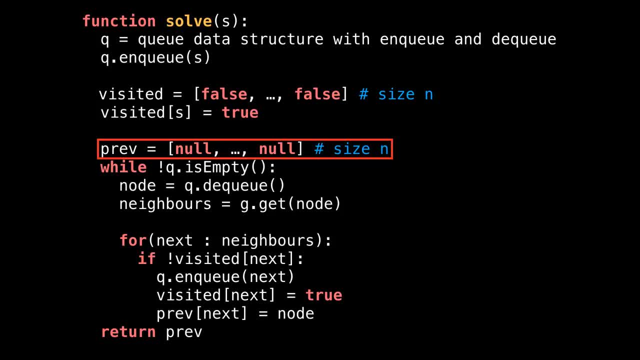 from the start to the end node. Initially, this array should be initialized with all null values. This array tracks who the parent of node I was, So we can reconstruct the path later. Let's loop while the queue is not empty and pull out the top node from the queue by issuing a dequeue operation, then reach inside the. 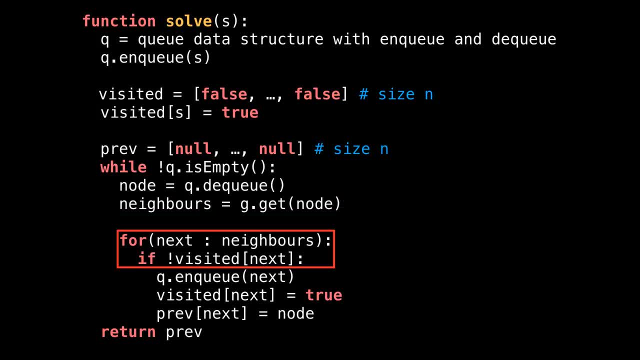 adjacency lists and get all the neighbors of this node loop over each unvisited node Once we find a next unvisited node and cue it to the queue market as visited and keep track of the parent node of the next node In the Prev array Once the queue is empty and our breadth first search is complete. 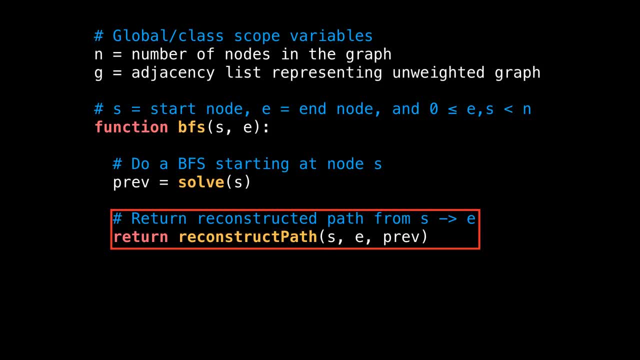 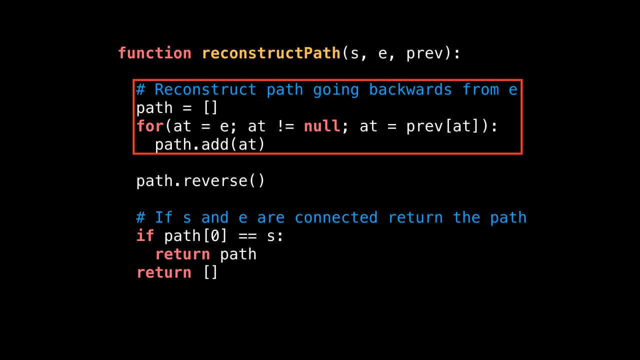 simply return the Prev array Back inside the breadth first search method, take the output of the solve method, which gave us the Prev array, and call the reconstruct path method. Here we are inside the reconstruct path method. The first thing we do is actually: 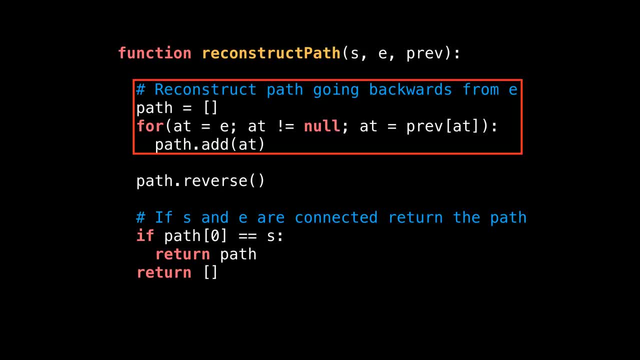 reconstruct the path by looping backwards from the end node And making our way back to the start node. that is assuming we can reach it. The reason the Prev array had to be initialized to all null values is because that is the way I'm checking whether or not the for loop should stop, Since we loop through the Prev array.